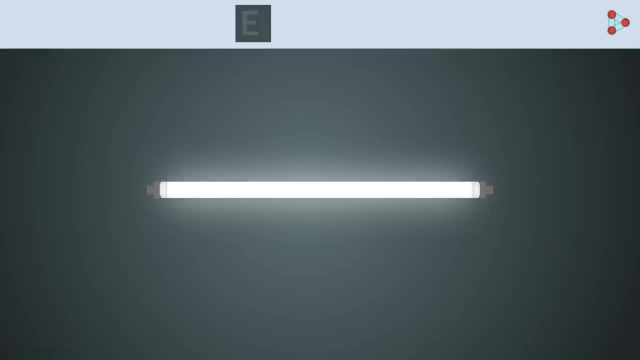 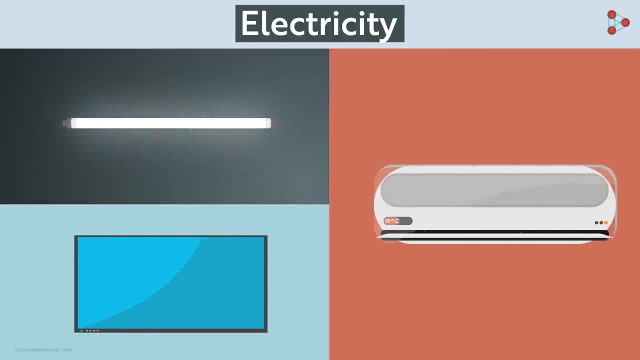 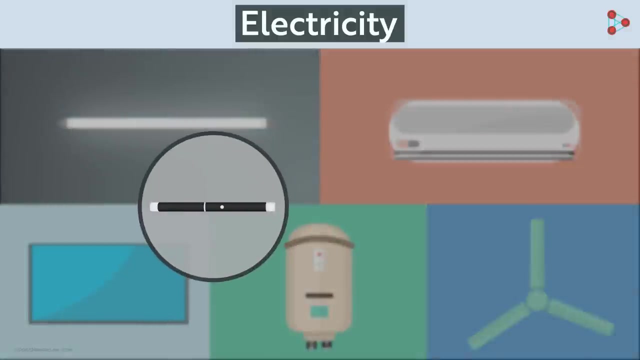 You must be aware of the fact that lights in our homes work on electricity. However, they are not the only ones that use electricity. Our televisions, air conditioners, water heaters, fans and so on also need electricity to function. Laser light or even small flashlights also work on electricity. 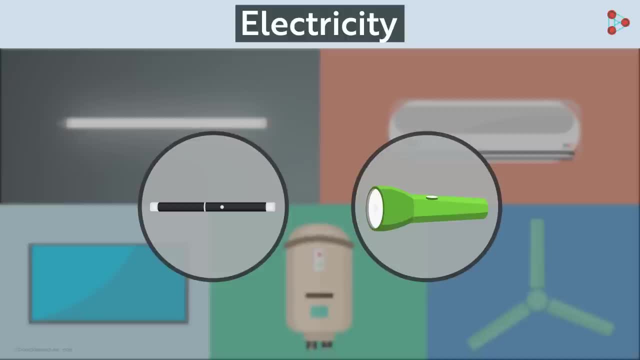 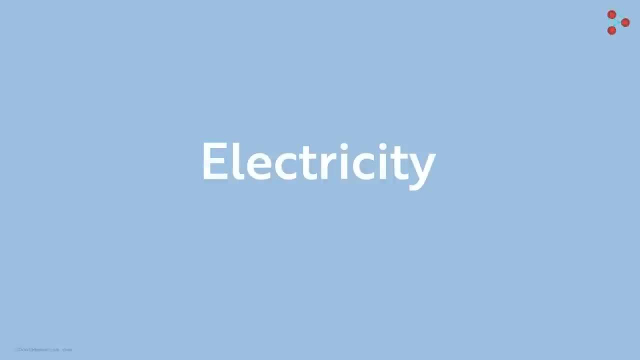 Imagine a life without electricity in the world today. The discovery of electricity has helped to start a new revolution in the history of humankind. But let's just keep aside all the rhetoric And try to understand the real thing. I haven't really told you what the term electricity means. 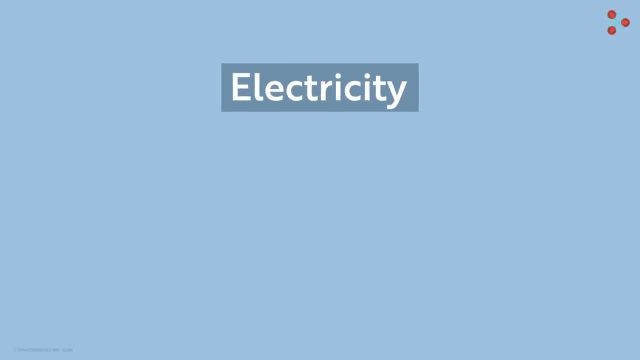 Well, there are basically two forms of electricity. One is static electricity and the other is dynamic electricity. For now, we are only interested in dynamic electricity. From the name itself, we can say that it implies moving electricity, or more precisely, moving electric charges. 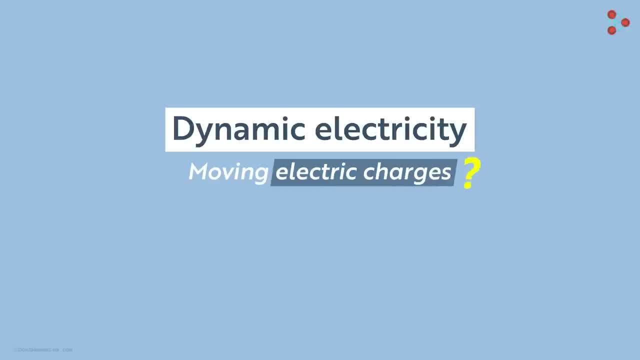 Now the next question you have will be: WHAT ARE ELECTRIC CHARGES? The concept of electric charges is very important in physics and it cannot be explained in a video or two, But I will still try to give you a short and to the point explanation of this concept. 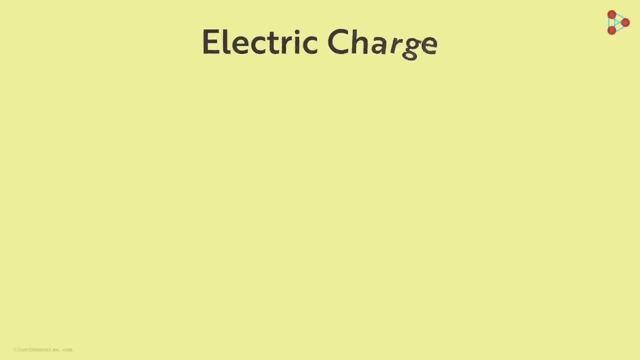 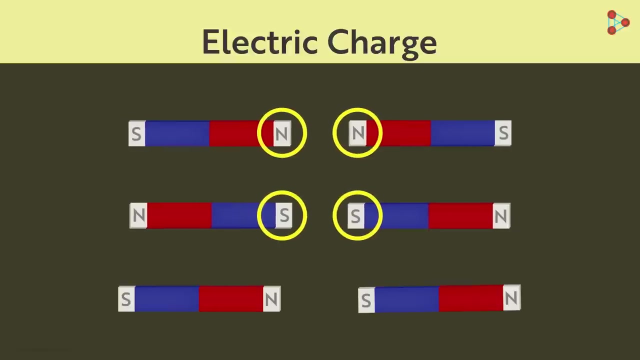 So let's begin. There are two types of electric charges: Positive, denoted by the plus sign, and negative, denoted by the minus sign. Think of magnets for a moment. We know that two like poles, that is, two north or two south poles of magnets repel each other. 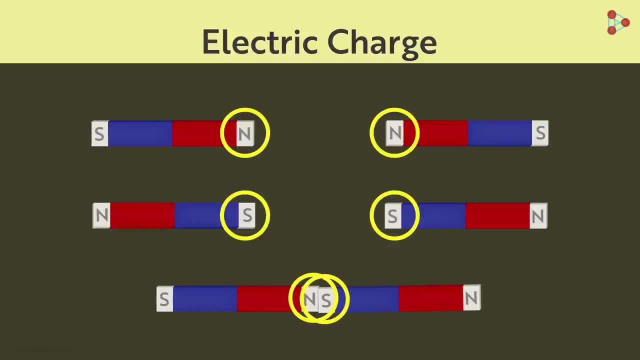 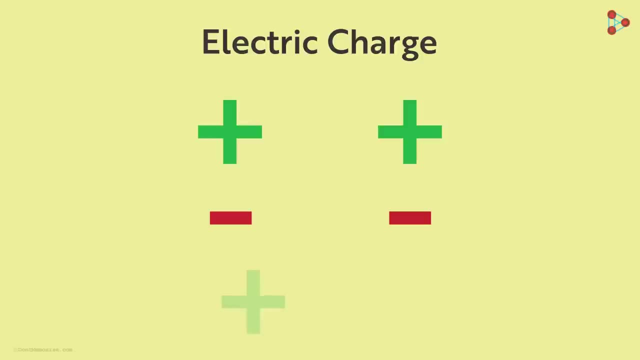 And, unlike poles, attract each other. Similarly, like charges, that is, two positive or two negative ones- repel each other and, unlike charges that is a positive and a negative one, attract each other. But what exactly is charged? 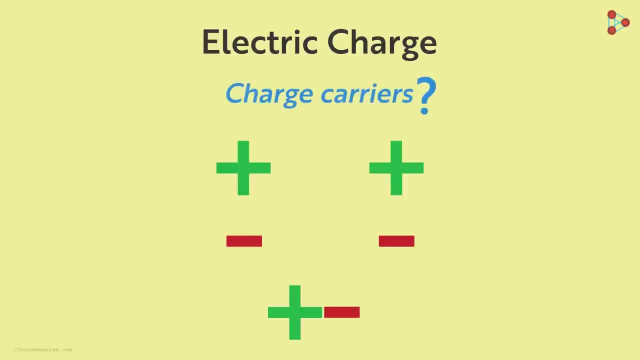 Or in other words, who actually carries these charges? Well, these charges are carried by tiny particles with incredibly small, very small mass. They are called subatomic particles. The positive charges are carried by particles called protons, while negative ones are carried by particles called electrons. 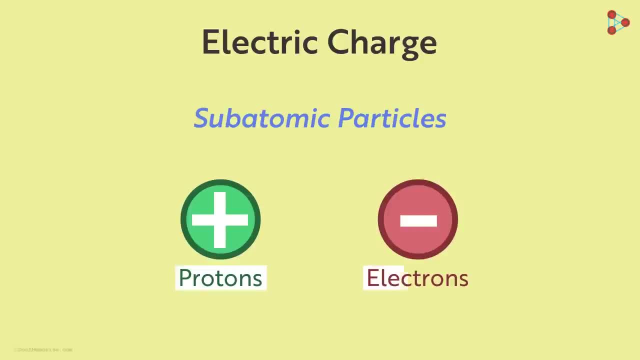 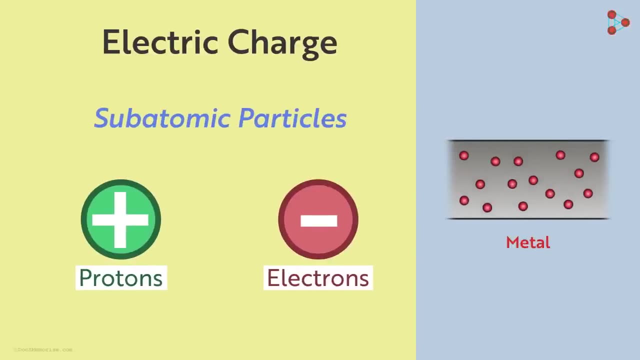 There are billions and trillions of protons and electrons present in any object around us. In some objects like metals, electrons can move randomly, While in non-metals their position is kind of fixed and hence they cannot move freely. Now any object like metals, electrons can move randomly.